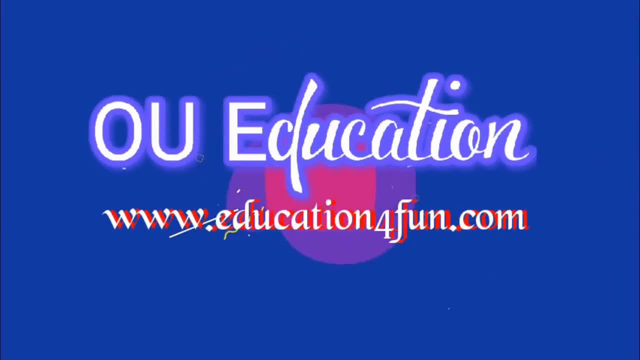 Hello guys, we are back with our next lecture. In this lecture, let us go through quality attributes. So quality attributes are given by this scientist, guys, So I cannot pronounce the name properly, So that's the reason why I'm skipping. So, in shortcut, he's called. 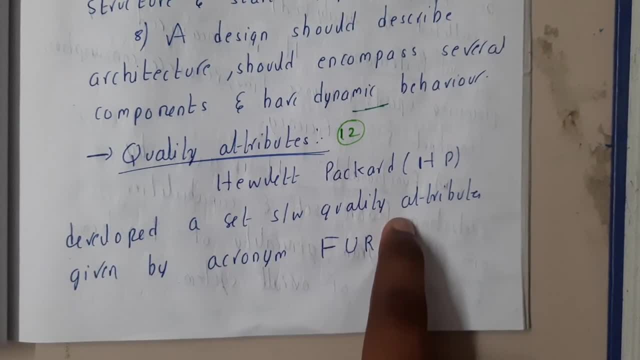 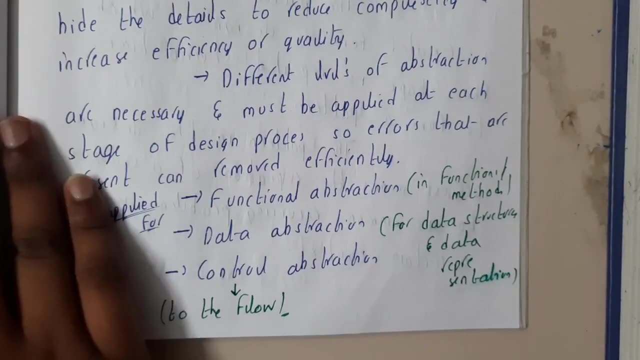 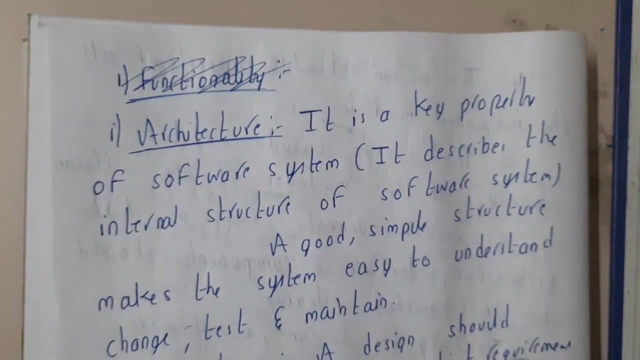 as HP, He developed a set of software quality attributes, Okay So, which are given by the acronym F U R, P, S. Okay, So now let us see what are those. So the first one is nothing but architecture. Guys, I didn't write in the order. If you want, in the order, F U R. 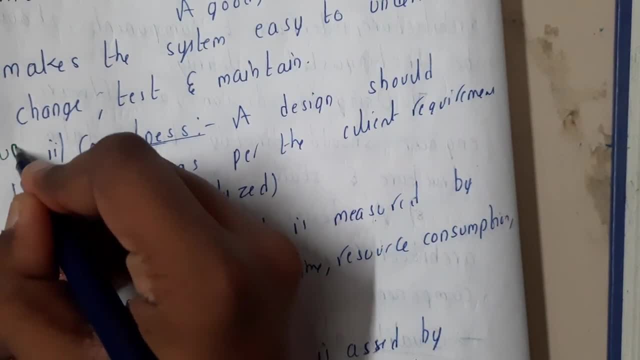 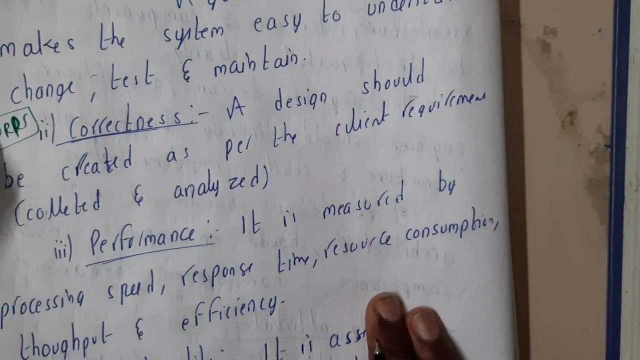 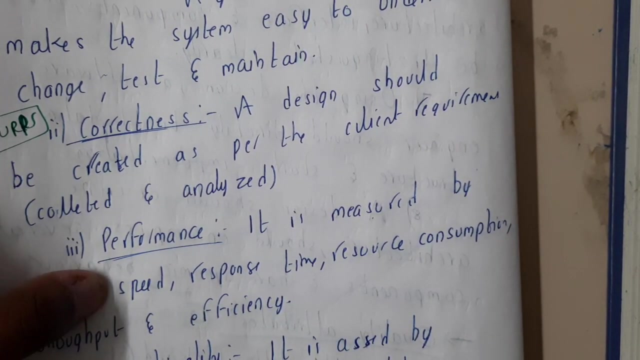 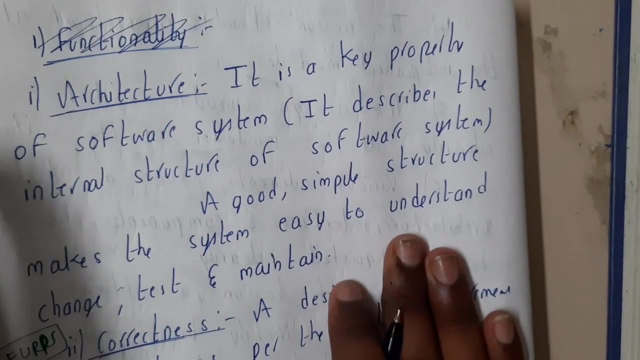 P S right, F? U R P S. Okay. So F means functionality, F? U means functionality, R means okay, P means performance. Okay, I think the letters does not match. I think so Okay, guys, let it be Okay. So. 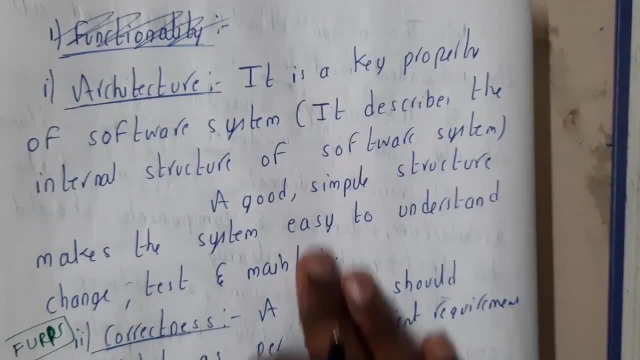 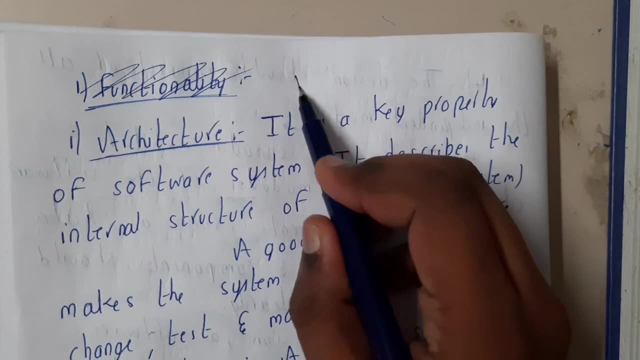 the first quality is nothing but architecture, guys, So it is a key property. So, basically, if you are designing a software module, even for smaller modules, we will be designing an architecture right. So it might be a data driven or content to flow like that There. 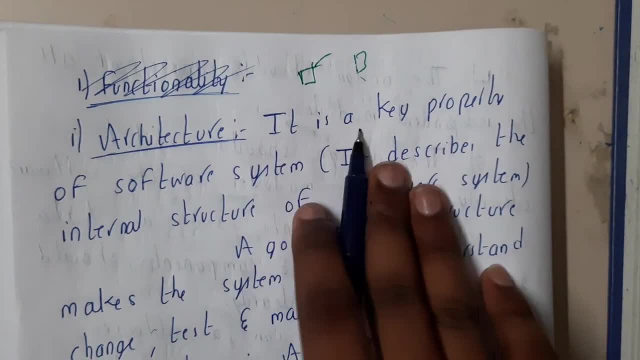 are multiple architectures, So we'll be following any architecture. So it is a key property of software system. It describes the internal structure of the software system, So it is a key property of software system. Guys, we'll be discussing about the architectures and 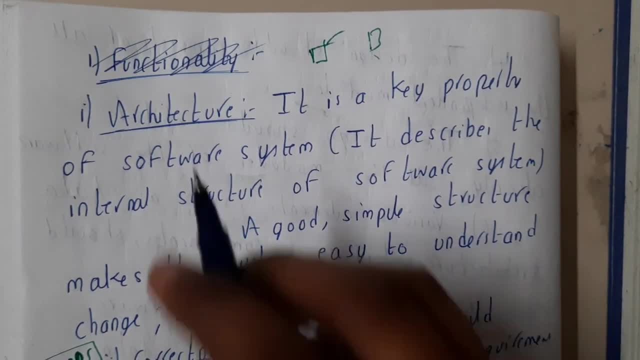 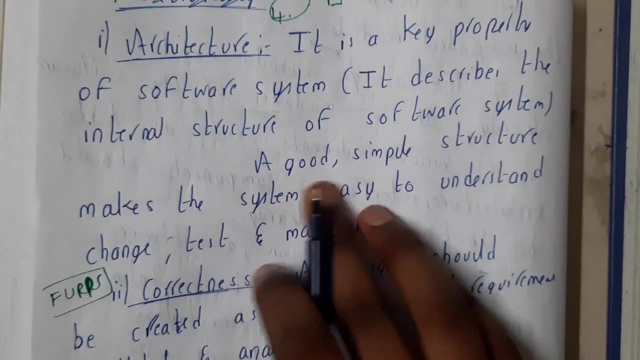 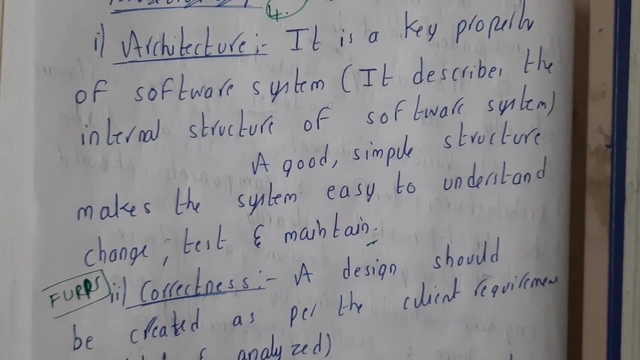 everything in the next unit, Like after around four to five units in 4.1 or 4.2,, we'll be starting the discussions about architectures, Don't worry, Okay. Okay, So a good or simple structure makes the system easy to understand and to changes and test and to maintain the. 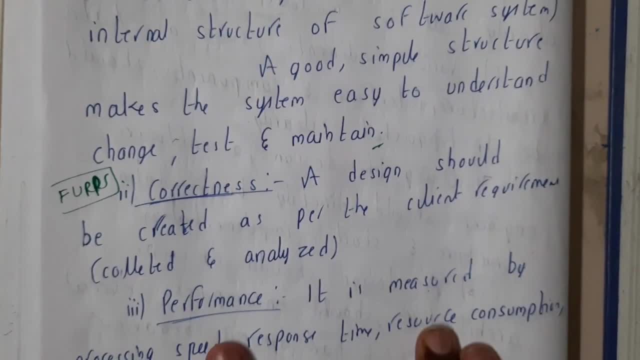 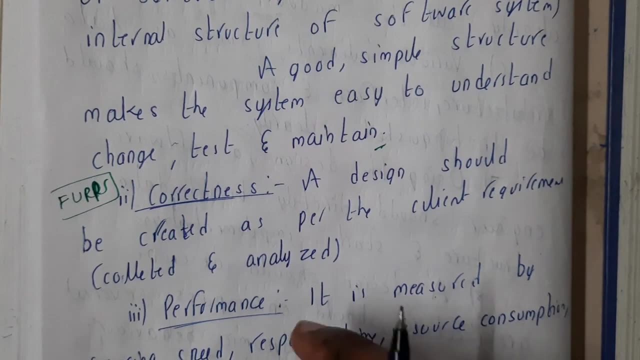 things right, So it makes everything easy and fast, guys. Okay, So the second is nothing but correctness, So correctness from the name itself we can say to check whether it is correct, Correct, Correct, Correct The client requirements or not. So a design should be created as per the client requirements. 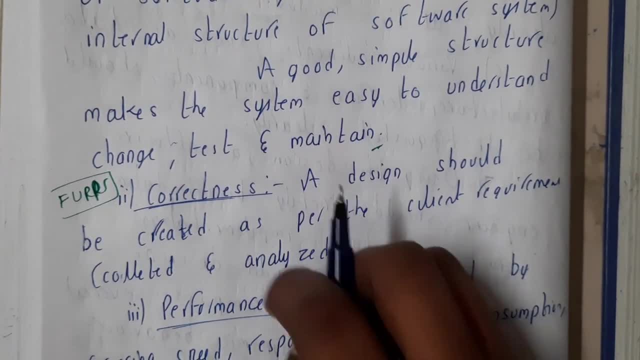 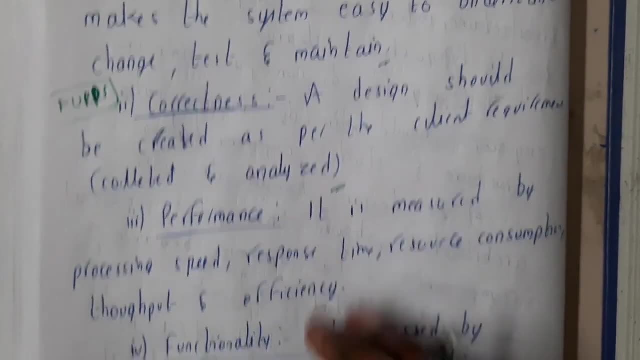 that are collected and analyzed. So it should be a hundred percent matching. So then we can say the software design or the design model is having the correctness, the property correctness. Similarly, performance, it is measured by the process speed, response time.